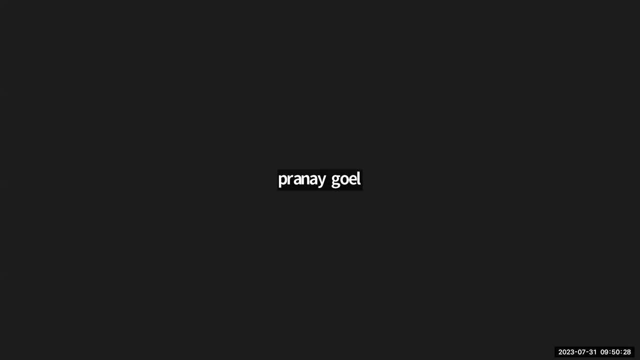 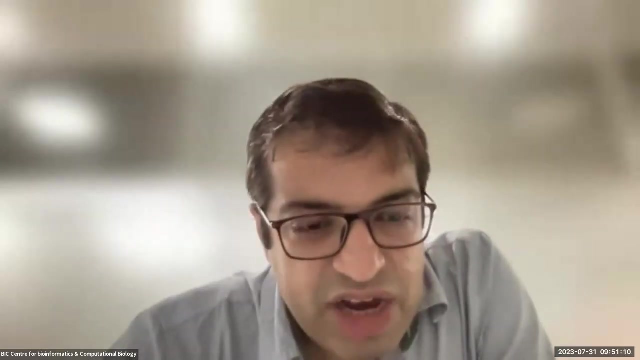 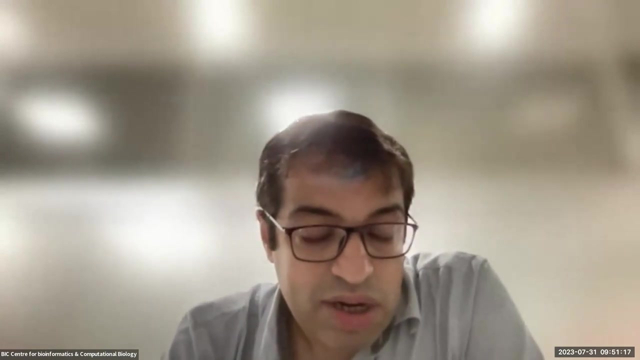 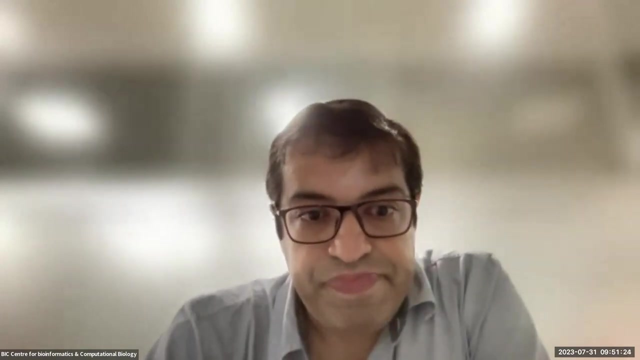 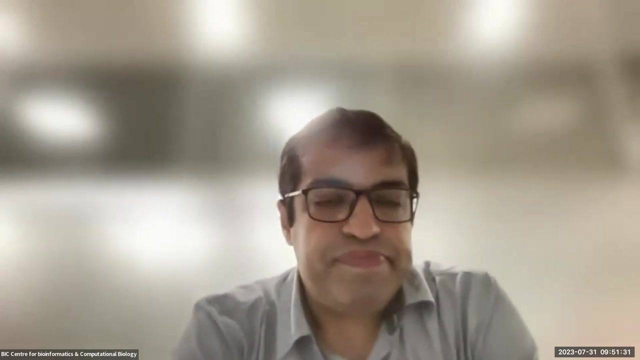 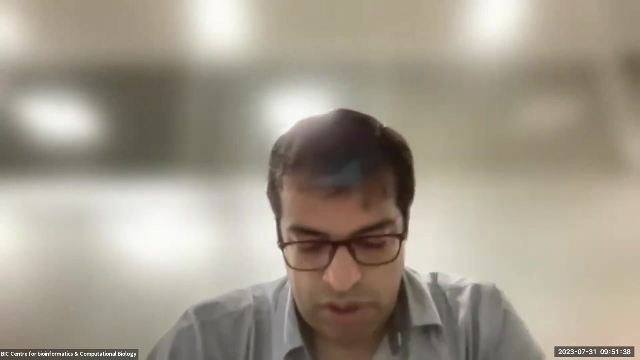 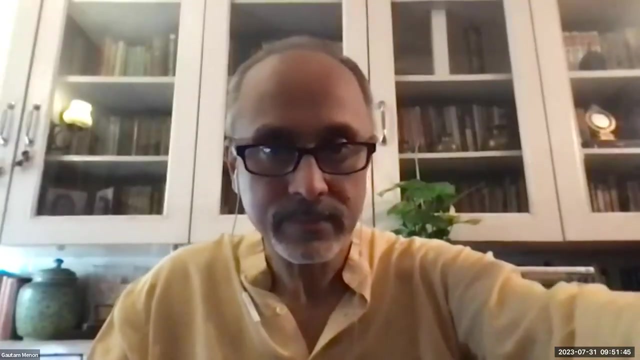 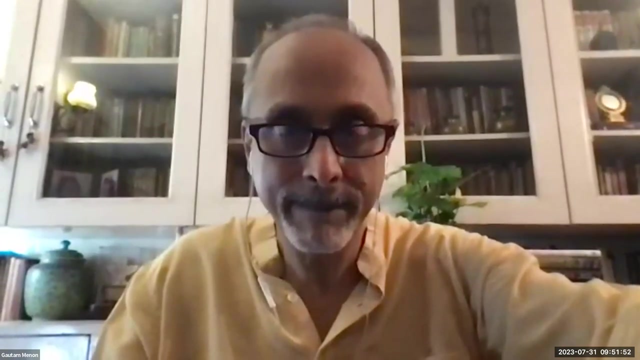 Thank you, And during the talk I request everyone to keep muted so that there is no echo or audio issues. Sir, I think we can start too. Sure, Want me to start. Should I go ahead? Yeah, I think so. 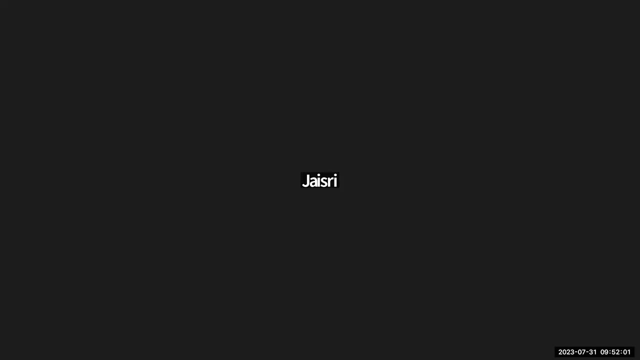 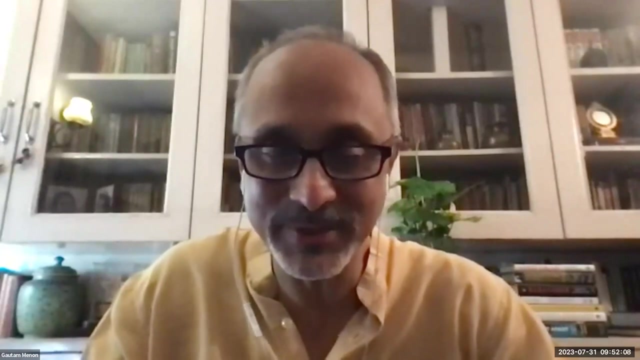 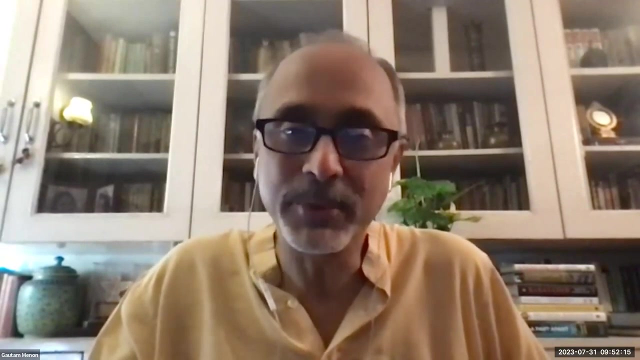 Okay, Recording is in process, I suppose. right, Ashish, I assume that all of you can hear me. So welcome to Ashoka University, in particular to the Center for Bioinformatics and Computational Biology at Ashoka University. This is a DPT-supported center that began about three years ago, roughly. 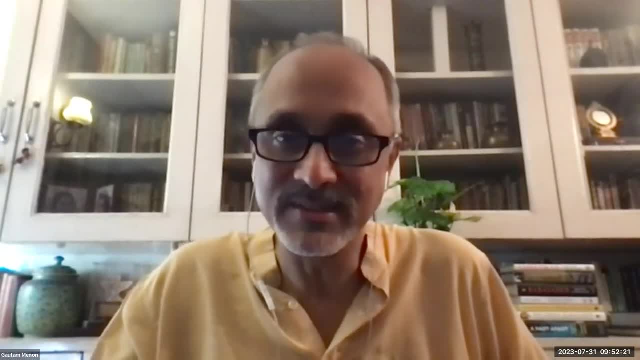 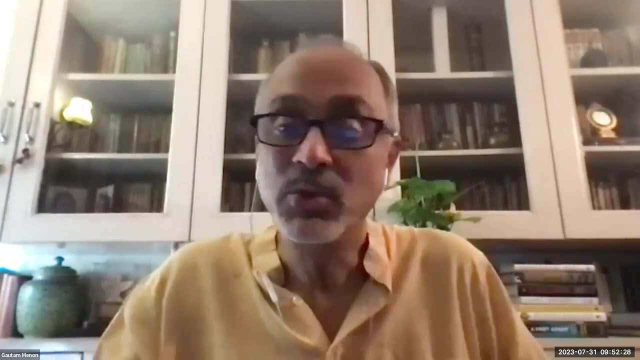 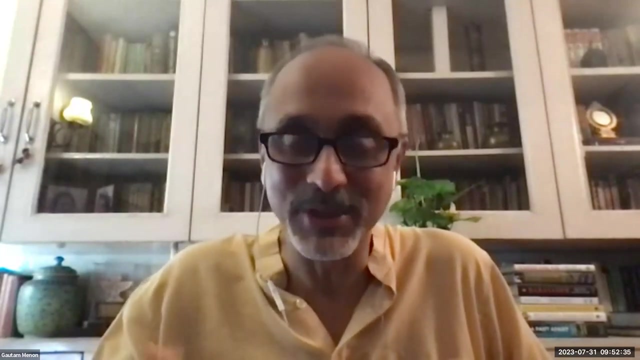 We do research, We provide services to campus researchers as well as outside, and another important part of what we do It is also teaching bioinformatics and computational biology to a range of students like you. So this is an online program. At some later point, presumably, it will become a truly offline program. We'll have you at Ashoka, as I understand those of you in Delhi who will be coming here on the third day to have a look on and how ideas and training from them can be generalized. So listen carefully. It's possible that you may not understand everything that they say, but there will be. time to ask them questions, There will be time to get clarifications from them And, of course, you can also follow up with them. Thank you, You can follow up with them at a later point, because these are all well-known people who. work within India. Just to quickly summarize the program that you have So soon you will be listening to Professor Pranay Goyal, who had the good fortune of meeting just last week at another meeting in Bangalore. Pranay is an expert in many areas, including physiology and type 2 diabetes. He will tell you about his own work on problems in bone aging in children, using deep learning. as I understand, After that there will be Professor Malay Banerjee. Malay Banerjee is a professor at the University of Delhi. He is a professor at the University of Delhi. 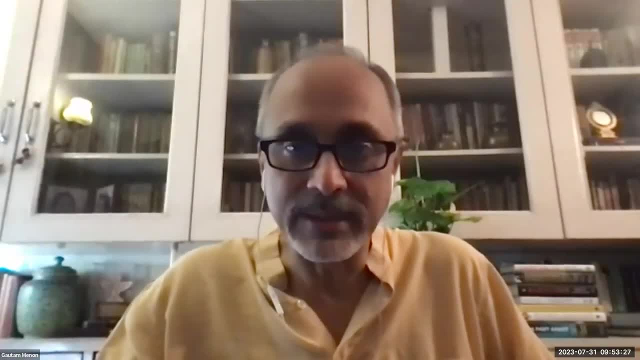 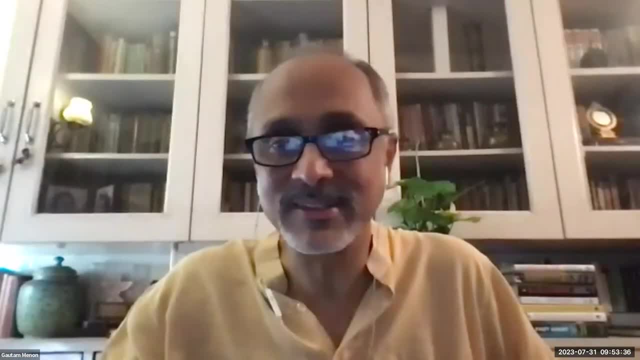 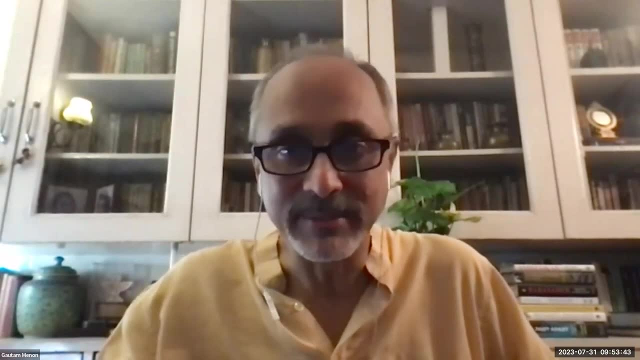 So that's again a different track altogether from the other stuff that you'll be hearing about. And then you have Vijay Krishnamoorthy, who is a physicist and biologist. This is today's program, and he will tell you about absolutely fascinating work that. 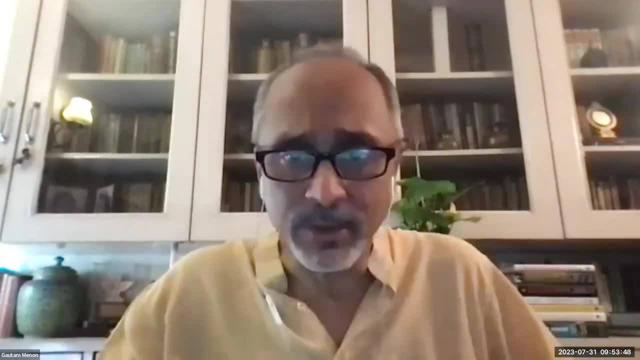 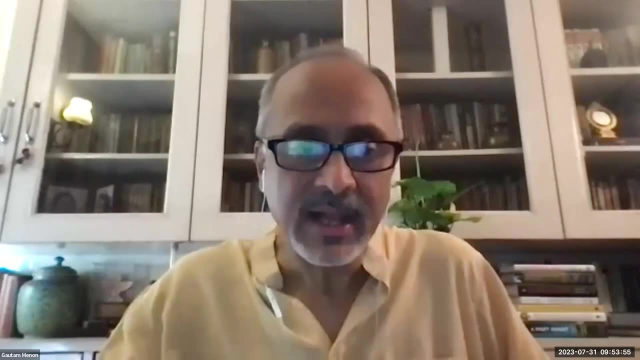 he's been doing on understanding how physics enters developmental processes. As I said earlier, these are not standard topics. These are not topics that you will hear pretty much anywhere. They're topics that can be considered absolutely frontier. So if you want to ask, look, I want to know what to do over the next 20,, 30 years. 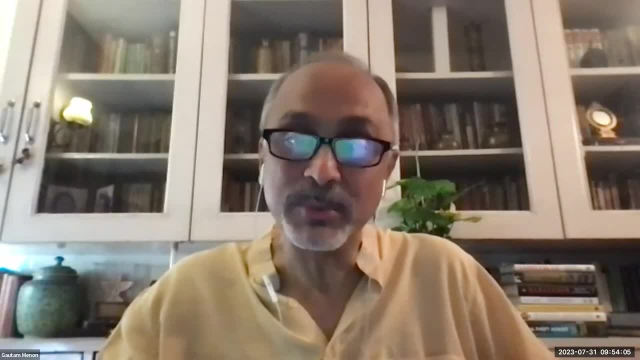 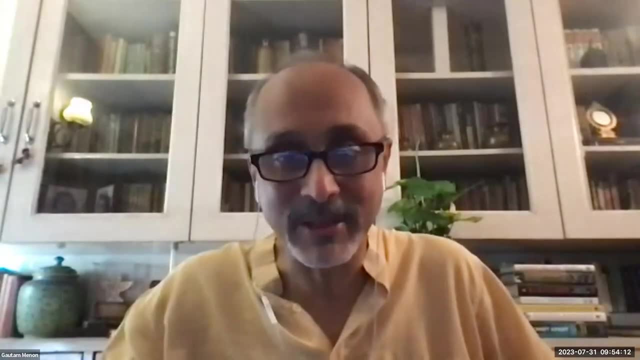 What are the topics that are going to be of interest to us, to people who work in computational biology and in bioinformatics, Not now, not yesterday, not three years ago, but over the next 5 to 10 to 20 to 30 to 50? 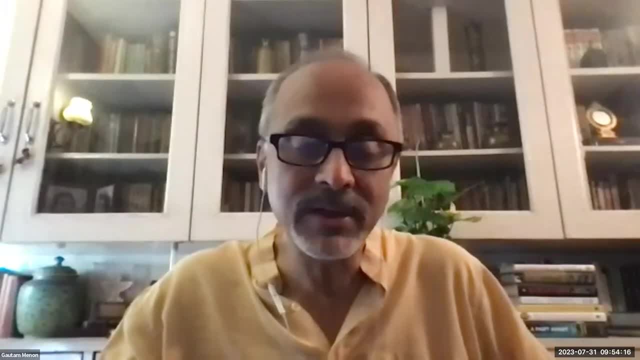 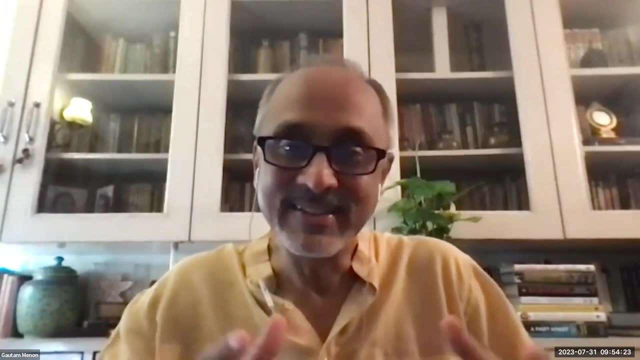 years ahead. These are the people that you should be listening to, And I will also look forward to hearing about them, hearing about what they do in this particular program, as I'm sure you will also be, And Ashish will be here. 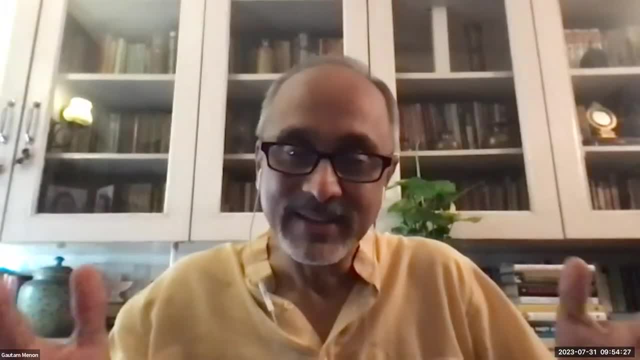 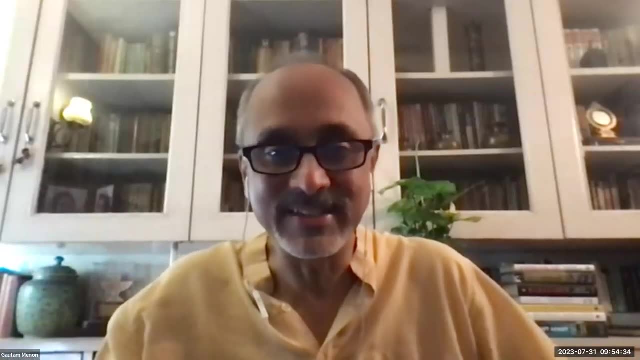 He will be here to help with anything that you might want. We have Deshri also here and they will help you both with the online and the later offline parts of the program. And let me just hand it back over to Ashish to take the program forward. welcoming all of you. 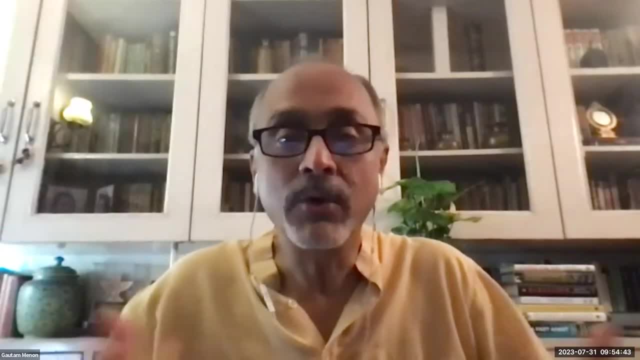 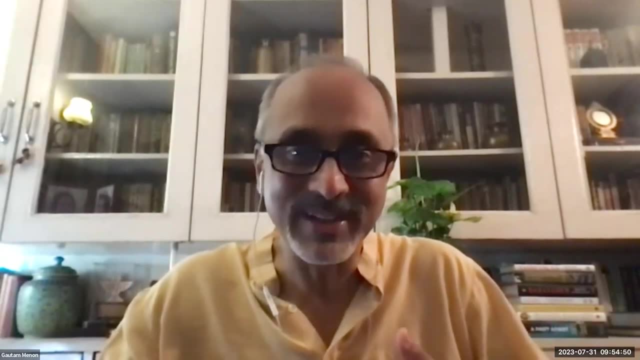 again. It's fun to see you. I hope we could all have met in person. Let me just extend Ashok University and the Bioinformatics Center for Bioinformatics and Computational Biology welcome to all of you. You will meet Professor Alok Bhattacharyya at the end of this, at the end of this program. 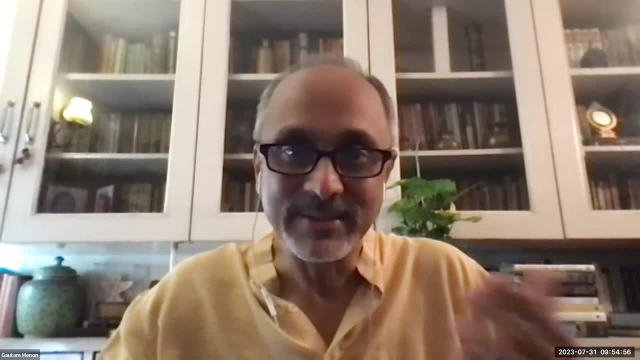 where he will thank all of you And provide you know, a sort of summary piece to everything that's gone on. But until then, enjoy yourself. Don't hesitate to ask questions and learn from everything that the speakers are telling you. Thank you, Professor Gautam Anand. 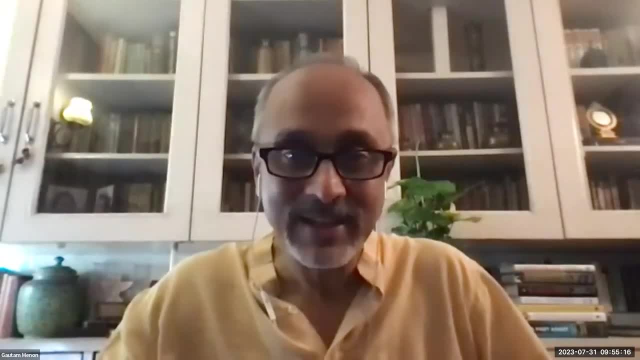 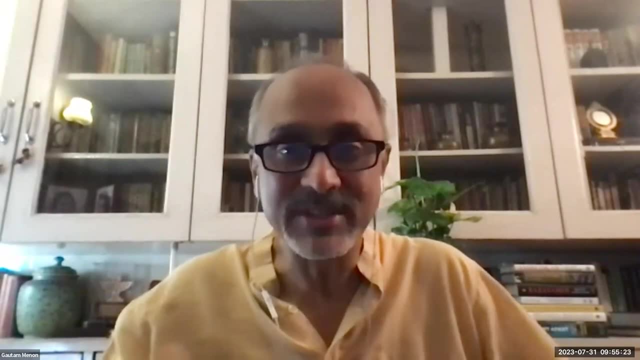 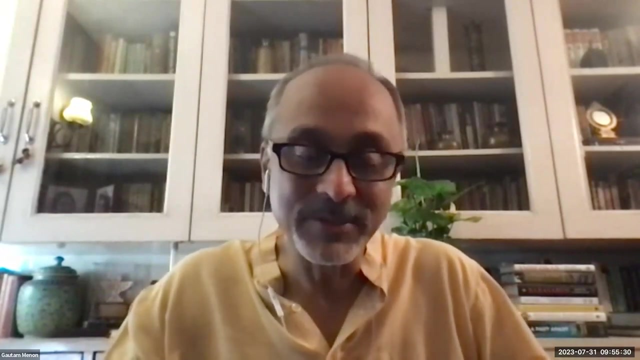 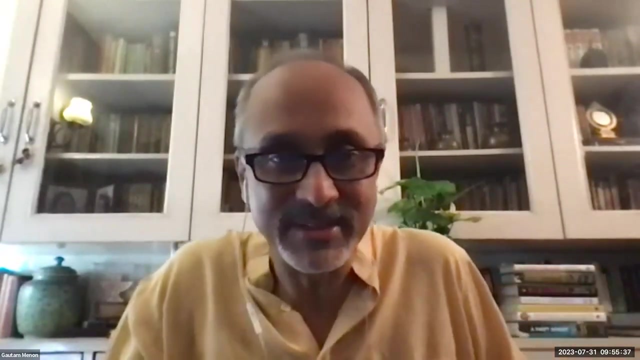 So I think all of you and I am very excited for these two days and I think we are a little early, but maybe we can get started with Dr Kanegoyal. Sure, should I begin? Yes, sir, Okay, wonderful. 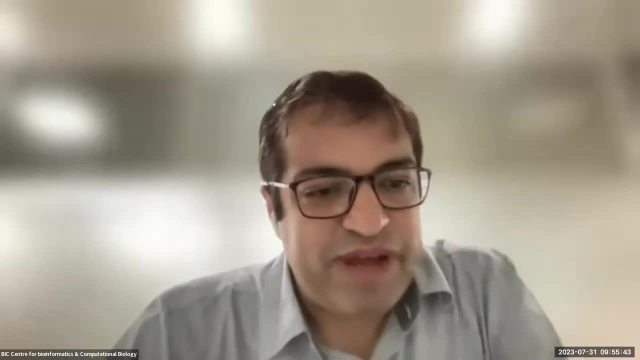 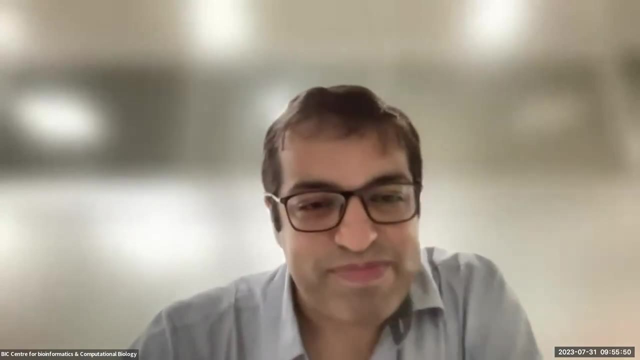 Yeah, just just a quick note that can everybody see the Q&A box. please don't like speak or keep. keep yourselves muted during the first 80 minutes And you can feel free to type your questions in the Q&A box as you hear the talk. 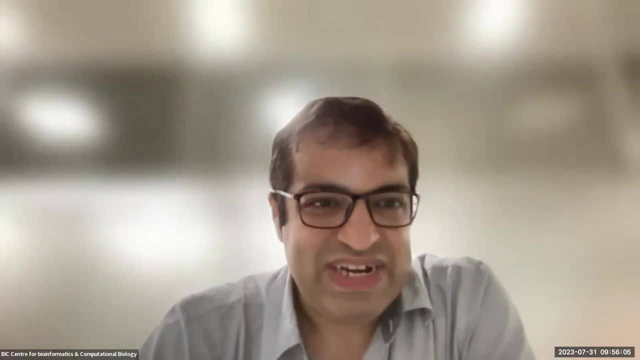 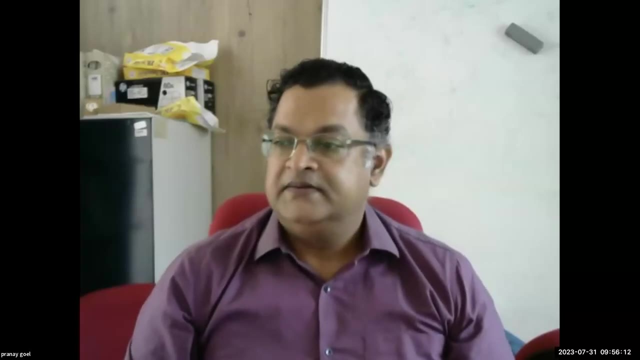 And then you know, after, in the Q&A section, in the last 10 minutes, I, or Dr Kanegoyal, will like call upon you one by one and you can ask questions. Okay, Thank you, Take it away, Dr. 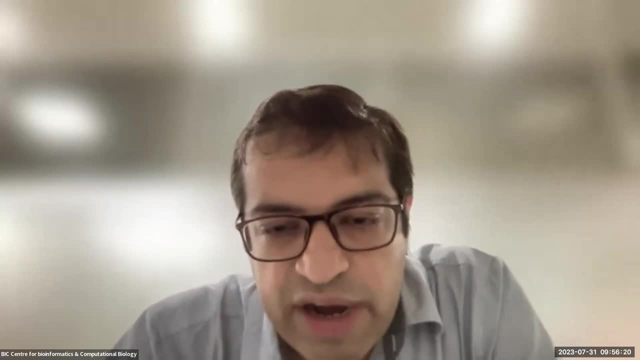 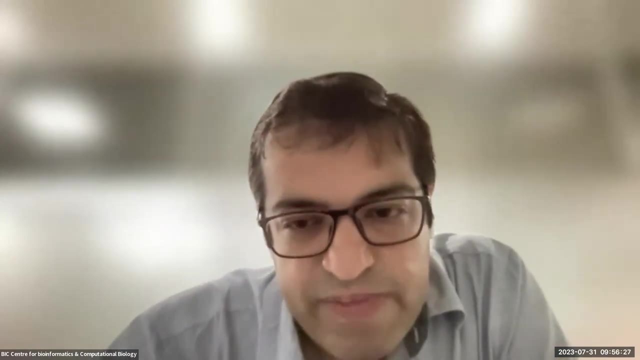 Gautam, Thank you very much. I hope you can hear me and at any time, if you don't see a slight change or if you can't hear me, please raise a flag and i will uh talk to you. uh, i'll try to fix it. 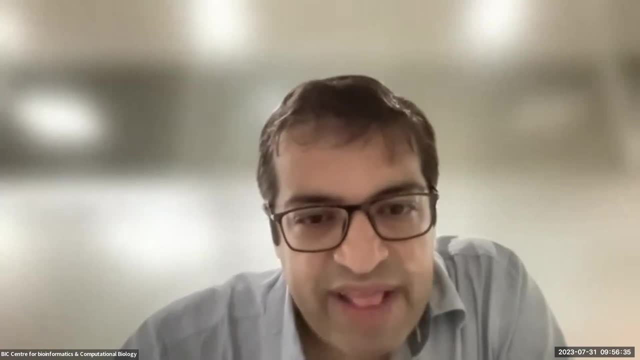 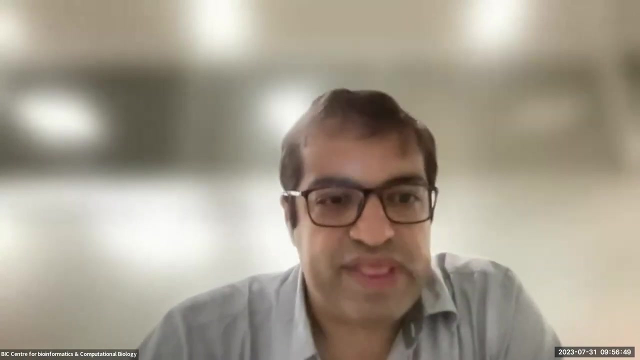 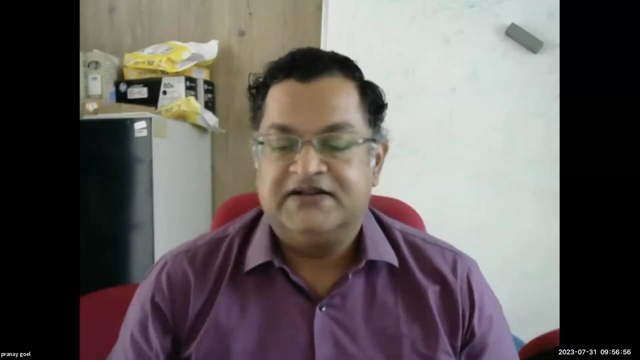 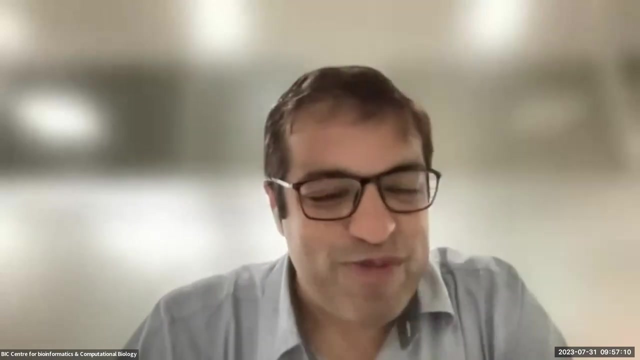 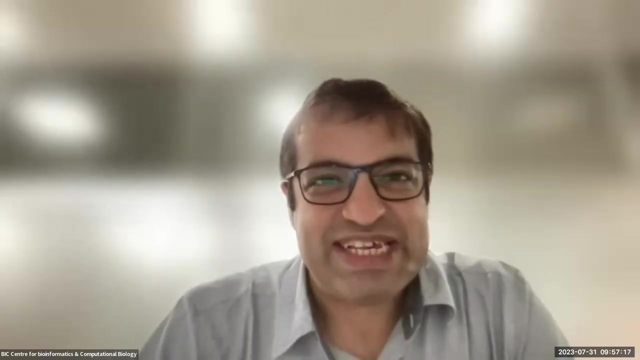 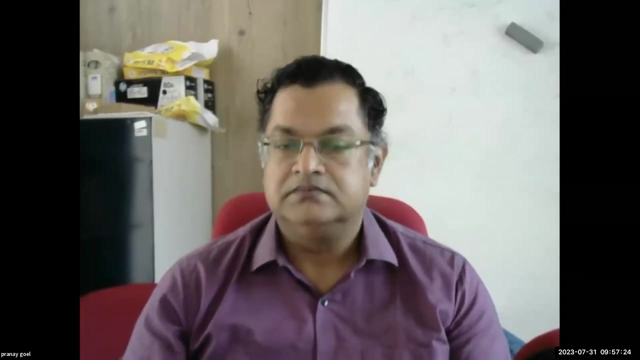 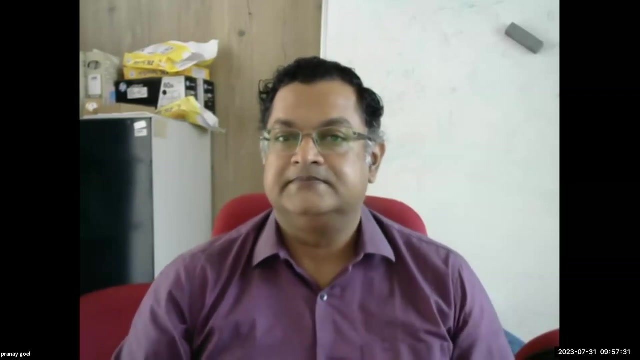 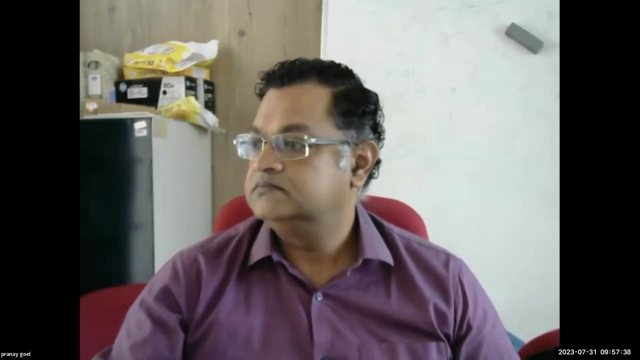 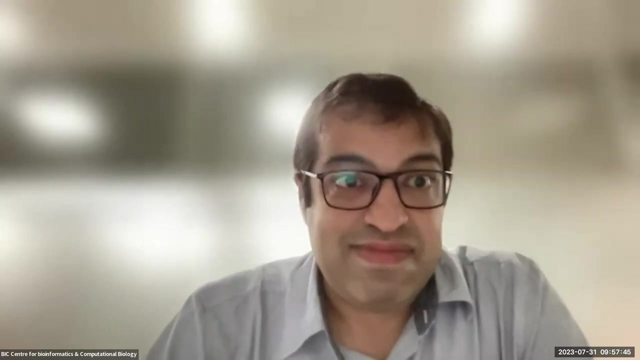 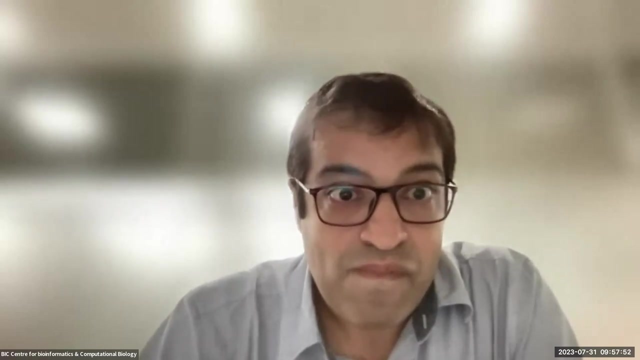 uh. so thank you very much for uh. sorry sir, sorry sir, i can't introduce you, my bad, so, oh, no, wait, okay, i shall do an introduction and then we can just give me a minute. just give me a minute. no, so, uh, in the mix up, so i wanted to introduce uh. 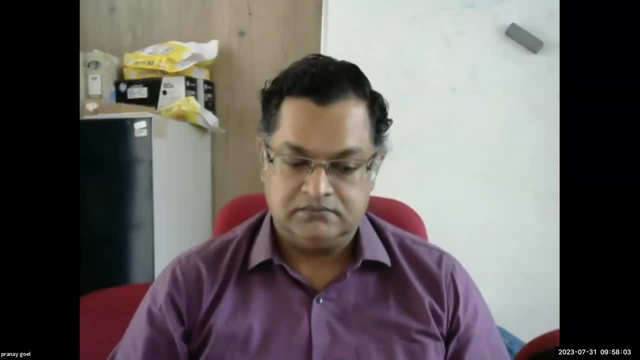 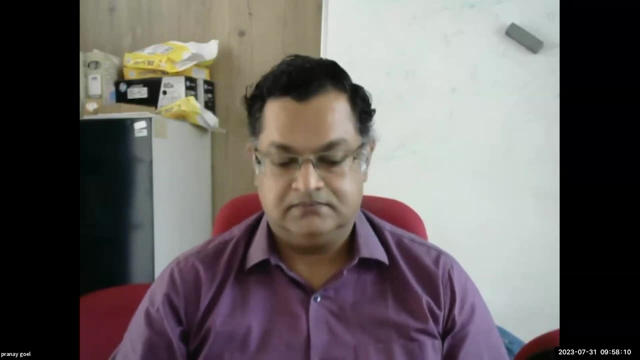 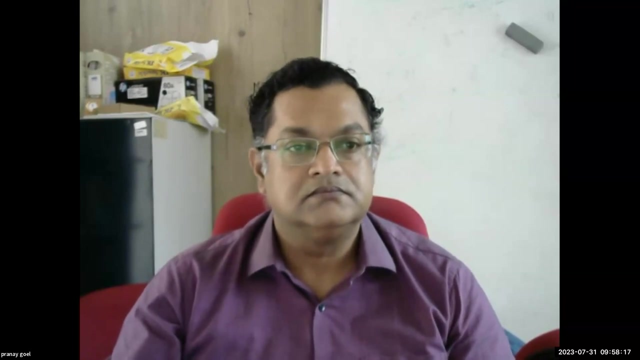 karen goel uh. professor carwell is an associate professor at icer pune. he is interested in studying biological systems using mathematically um analytical computational algorithmic approaches. his main focus areas are mathematical physiology and type 2 diabetes. he's also interested in data science and predictive modeling. 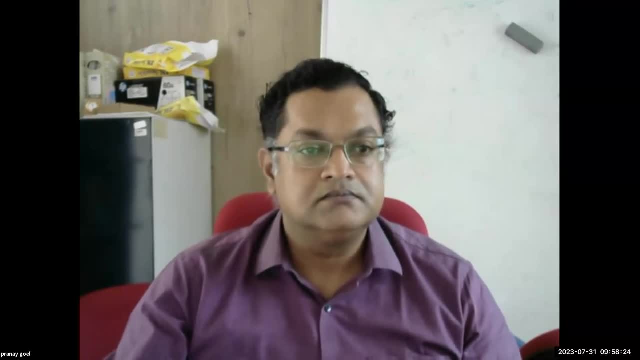 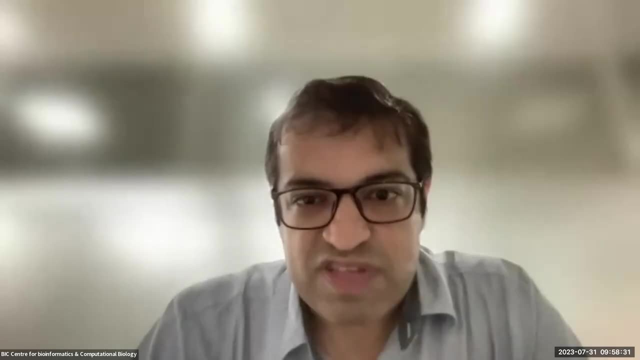 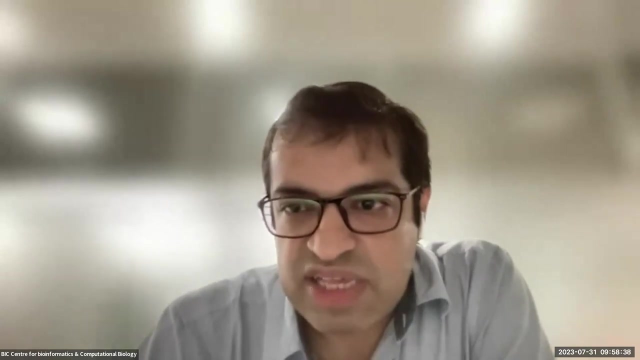 for healthcare and precision or personalized medicine. yeah, sorry for the mix-up. thank you very much for the introduction. uh, i'd like to begin by uh thanking gotham and alok and all of the other organizers for inviting me uh for to this, uh, to this workshop. 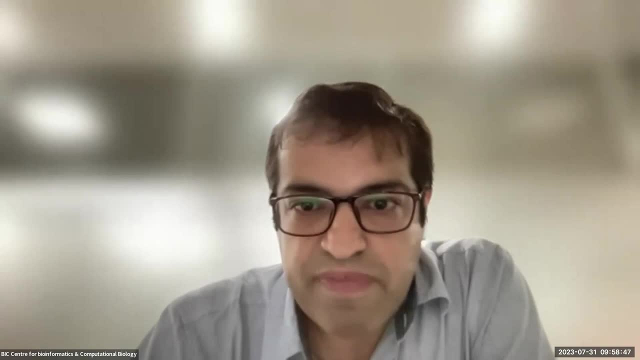 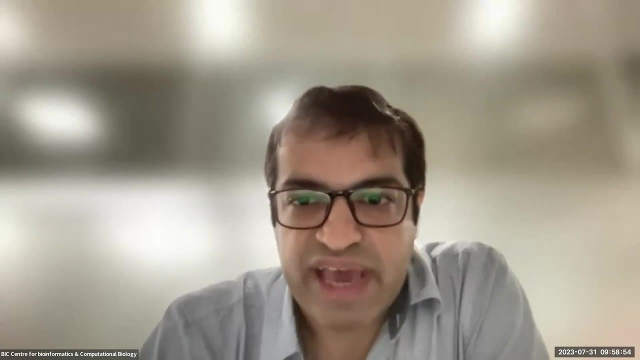 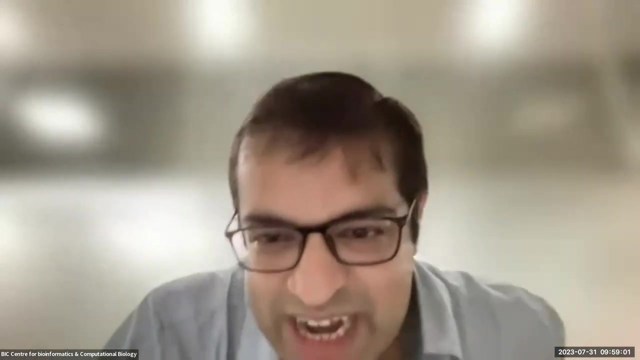 uh, i, i'm, uh, it's a. it's a great pleasure for me to be giving this talk to you. uh, there's a lot of uh very interesting fresh results that uh, you know, we've generated over the last uh couple of weeks and you know, much of this is actually a lot of this has been written up, a little bit of it towards. 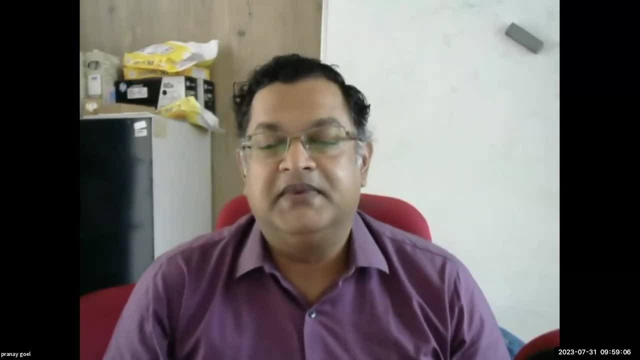 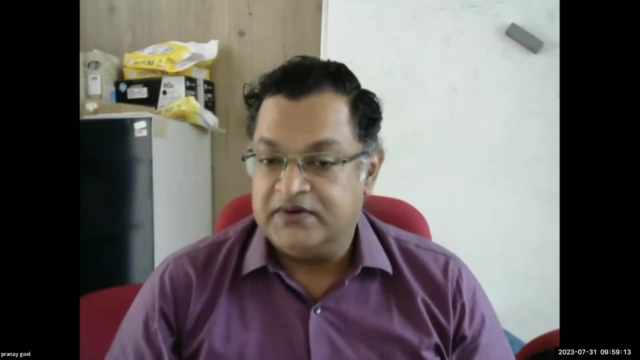 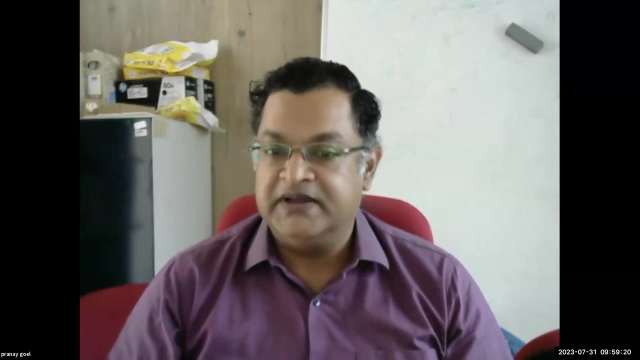 the end of the talk you'll see has yet to be sent out. so these are really truly very fresh results and I'm looking forward to getting your reaction on these ideas. So, as I understand, there's a number of students in the audience. is that correct? 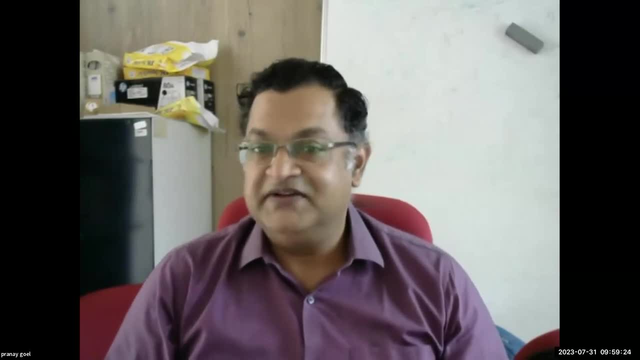 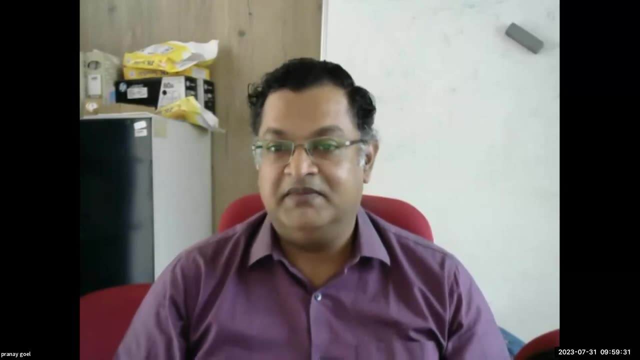 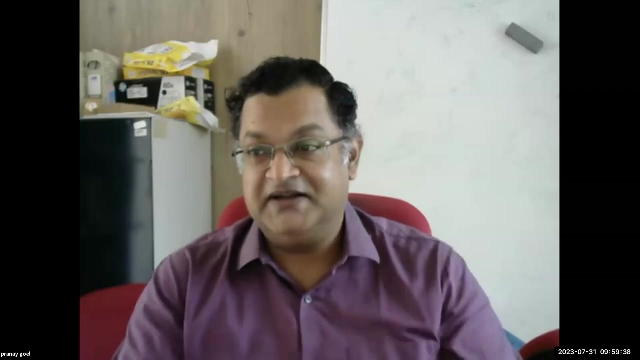 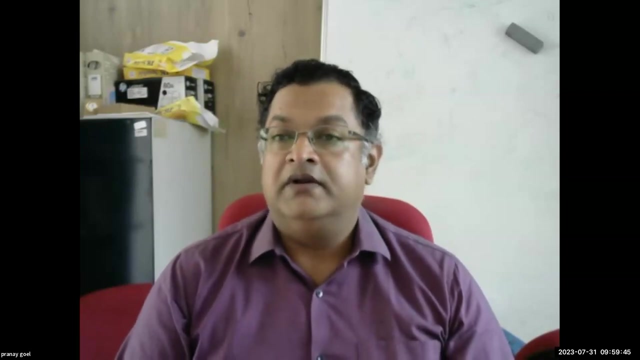 I think they're all students, Pranay. Oh, okay, Wonderful, Good to know. So I will try to keep my talk at a level where students can follow along And if you have any questions, please interrupt me either directly by raising a hand or through Arshiv or Gautam, or maybe someone can moderate it, the discussion. 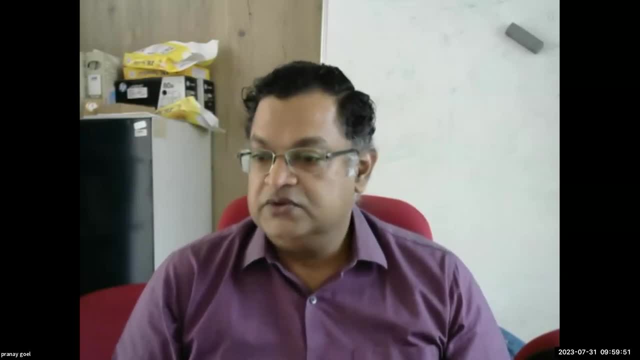 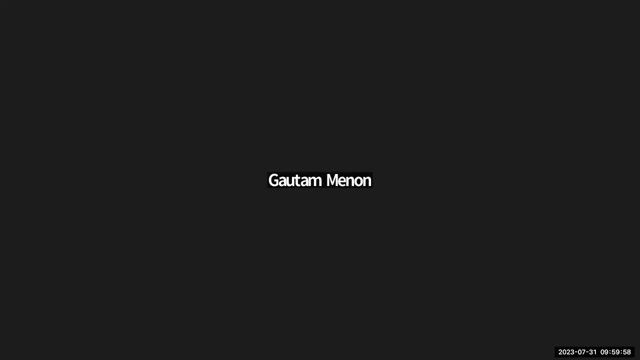 But I'm very happy to answer any questions. The talk duration is about 60 minutes or so And I would like to leave plenty of questions, plenty of time for questions and answers and any discussions that you might want to have. I appreciate it. Thank you. 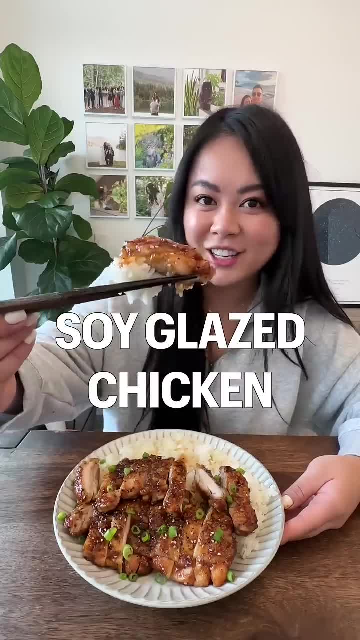 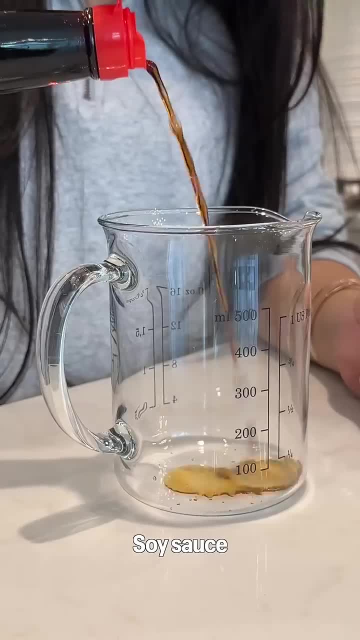 Back with another 20-minute recipe. the best soy-glazed chicken: Season the chicken with salt and pepper, Coat the chicken with a thin layer of cornstarch. The sauce is super easy. Soy sauce, oyster sauce, honey, five-spice powder. 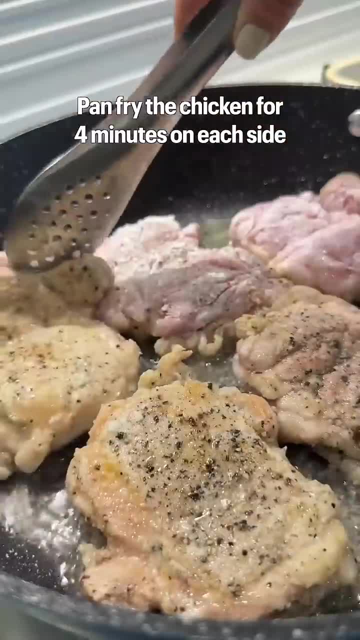 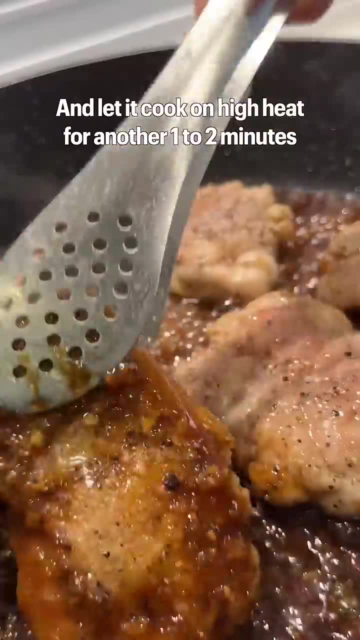 and a lot of garlic. Mix together. Pan-fry the chicken for four minutes on each side. Remove and set aside, Pour in the sauce, Let it simmer for 30 seconds, Add back in the chicken and let it cook on high heat for another one to two minutes. 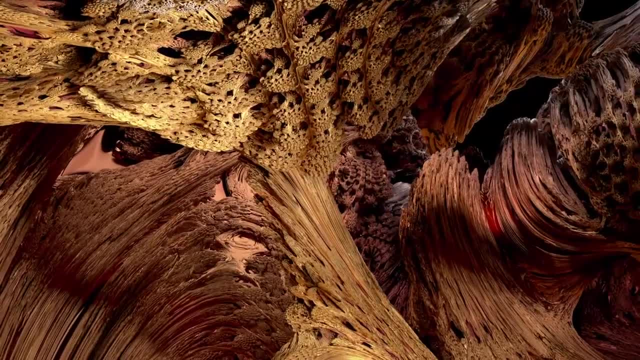 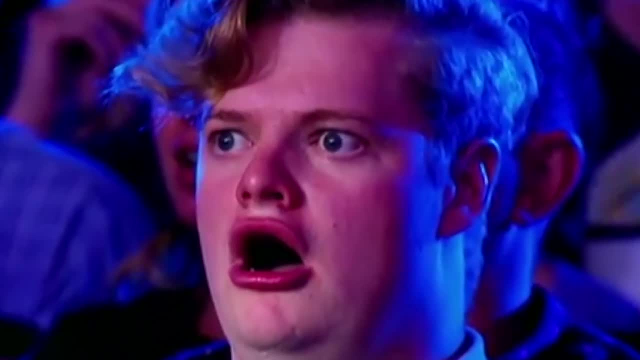 This awesome looking shape is called a mandel bulb. You could keep zooming into it literally forever and would still find new things, Only really limited by the speed of your graphics card, and this isn't the only one that exists. All it takes are some maths and you can make a huge. 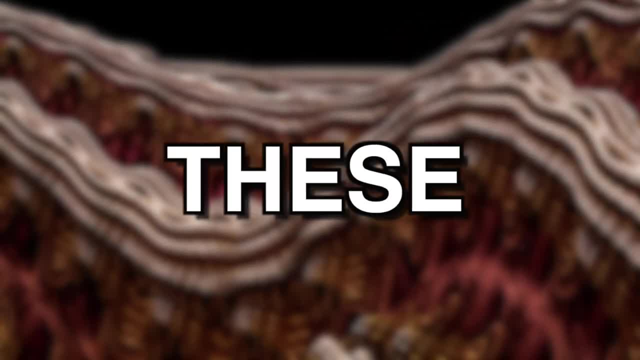 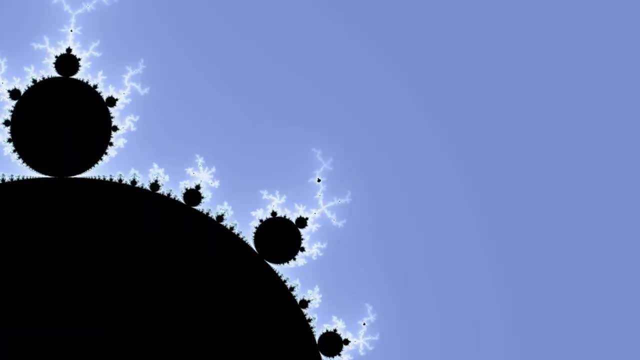 variety of different 3D fractals like this one. So where did these come from? In 1980, Benuit, Benuit, Benoit Mandelbrot Discovered the infinite 2D fractal called the Mandelbrot set Fast forward.